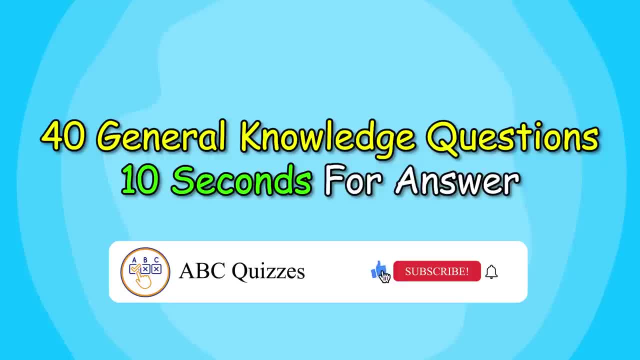 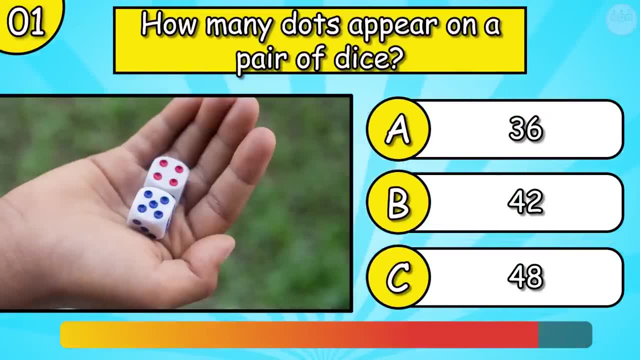 Hello ABC quizzers. In today's quiz you'll have to answer 40 general knowledge questions. Don't forget to subscribe to the channel so you won't miss new uploads. Let's start. How many dots appear on a pair of dice? In what country was Elon Musk born? Which is the only body part that is fully grown from birth? What animal produces pearls? Which country is the capital of Havana? Havana is the capital of what country? In which year did Usain Bolt set his 100-meter world record? 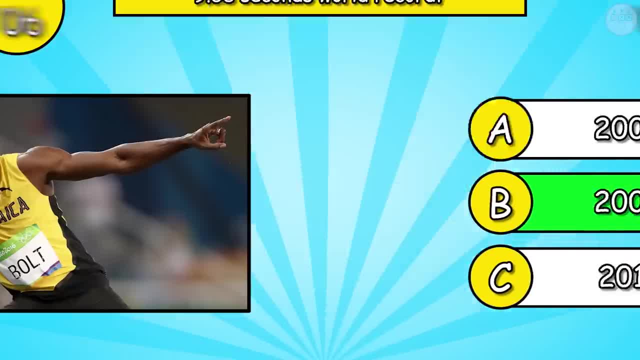 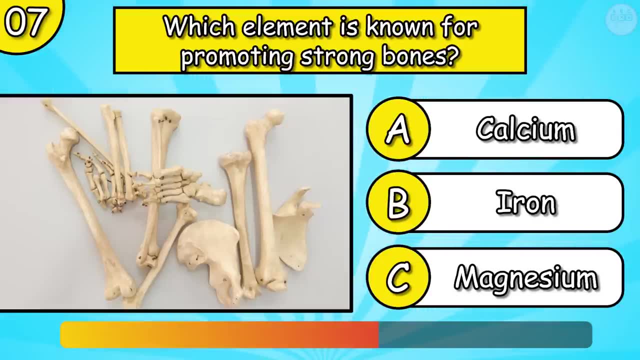 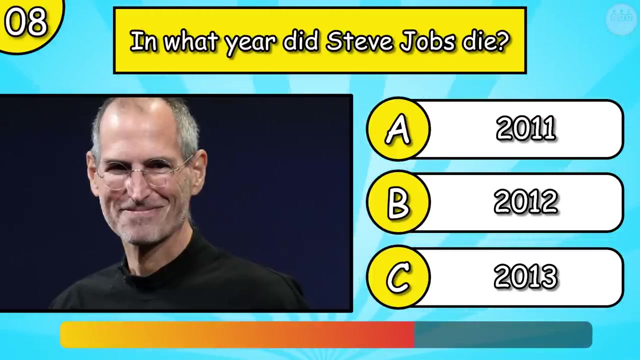 In which country was he born? Which element is known for promoting strong bones? No one knows this, but it can be difficult. How much does a needle track a bone Three meters? How much does a scale measure Three meters? What's the size of the tongue? 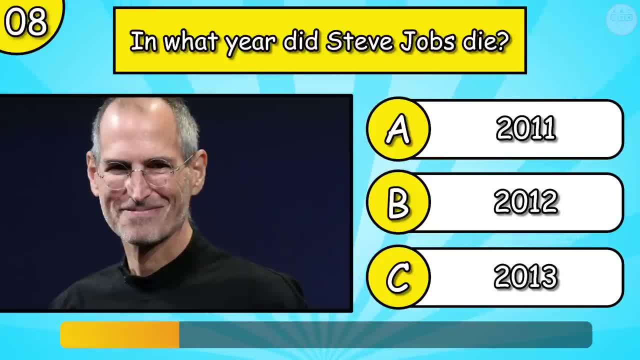 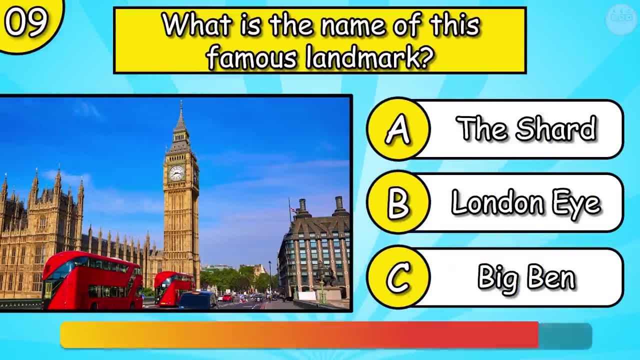 Three meters Right, Like this, And on tongue Like this, Like this, Like over here. Let's go to the next. Which was the answer? Las Las…. Las Las Las, What's the name of this famous landmark? 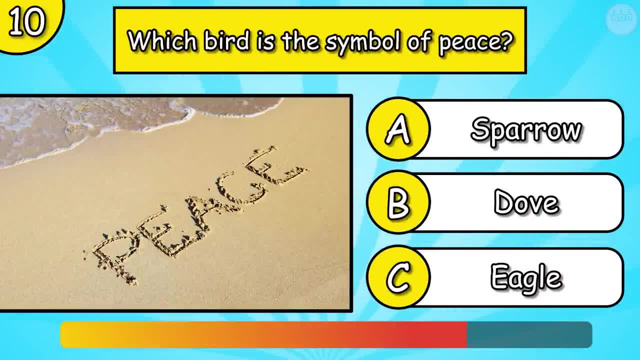 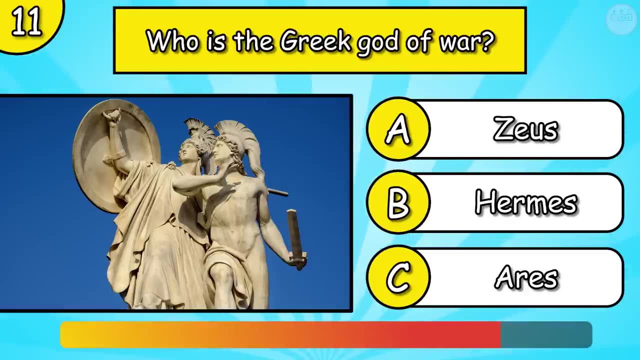 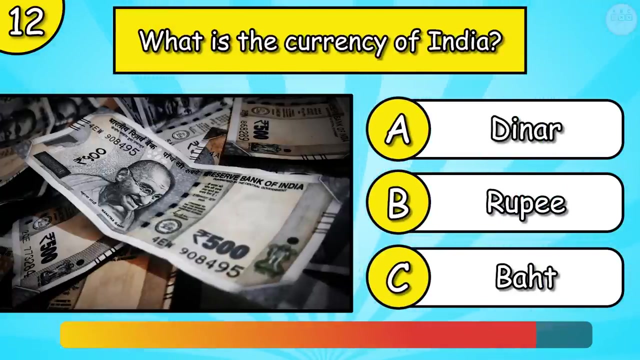 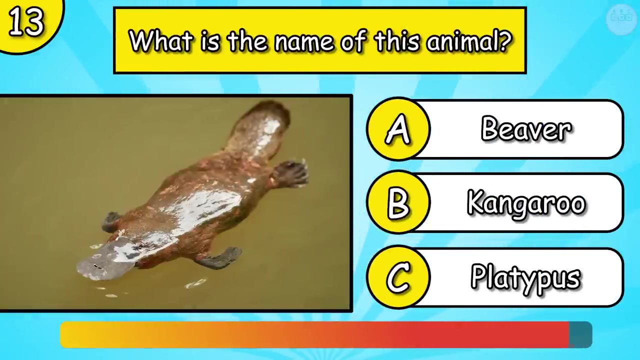 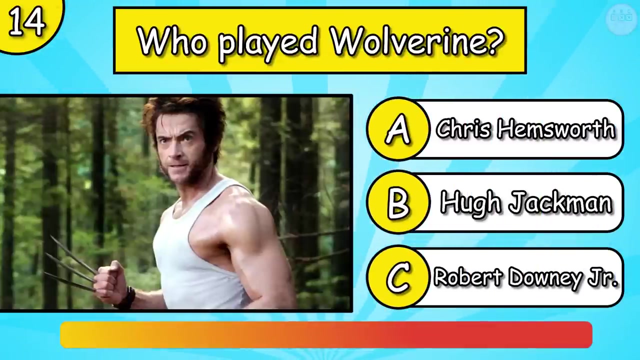 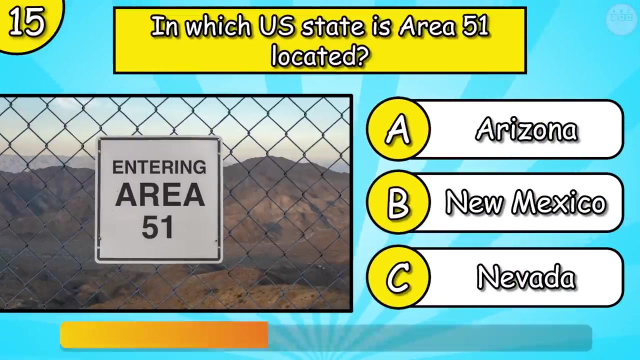 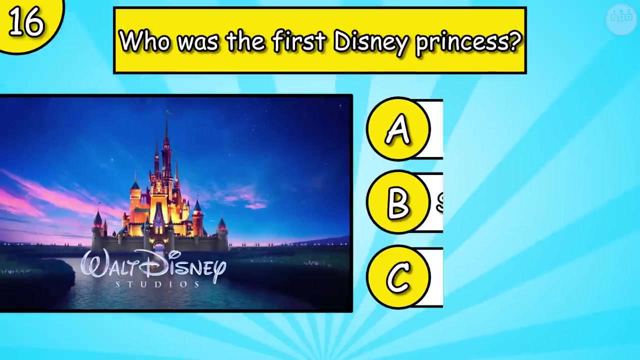 Which bird is the symbol of peace? Who is the Greek god of war? What is the currency of India? What is the name of this animal? Who played Wolverine? In which US state is Area 51 located? Who was the first Disney princess? 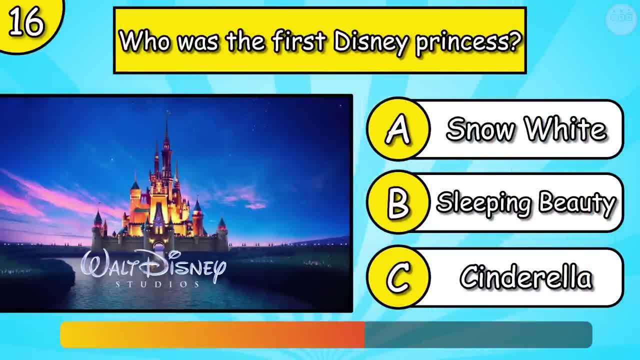 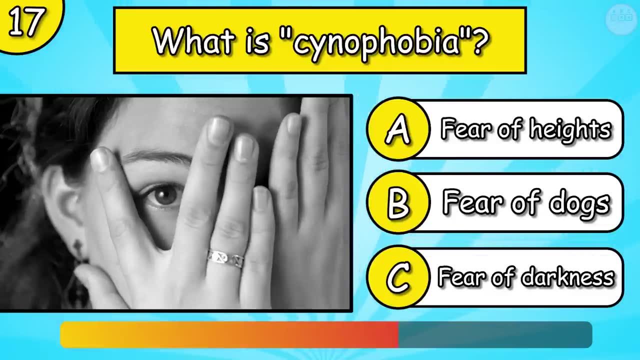 Takeout: What is xenophobia? You may have chosen either of these two Systems. What is xenophobia? Which of these email services is owned by Microsoft's Microsoft Scenario? Which of these email services is owned by Microsoft? You can choose them as follows. as following: 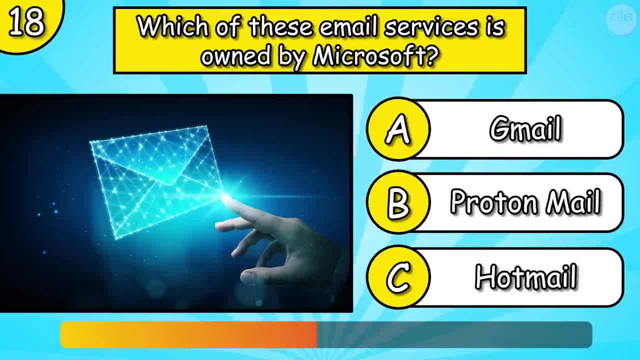 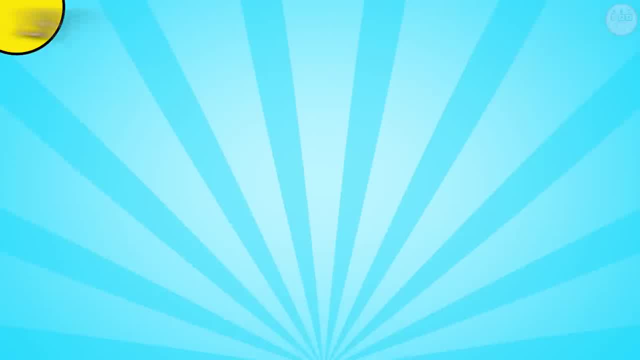 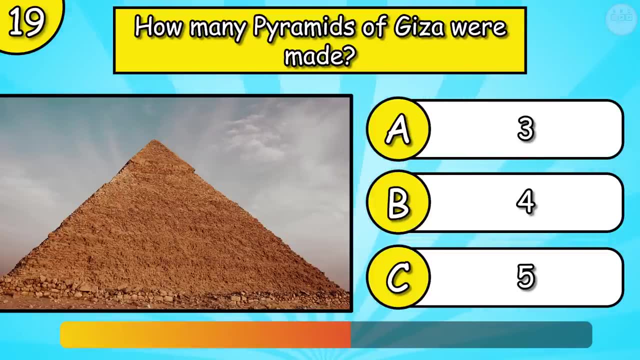 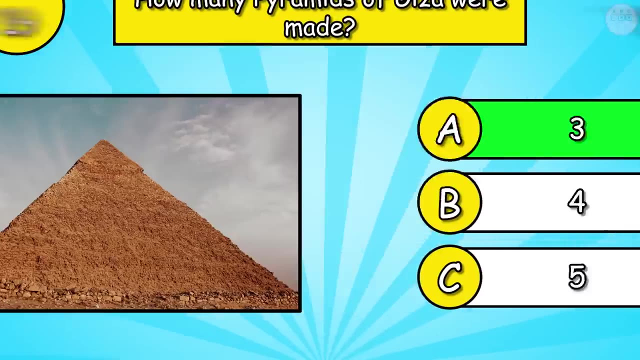 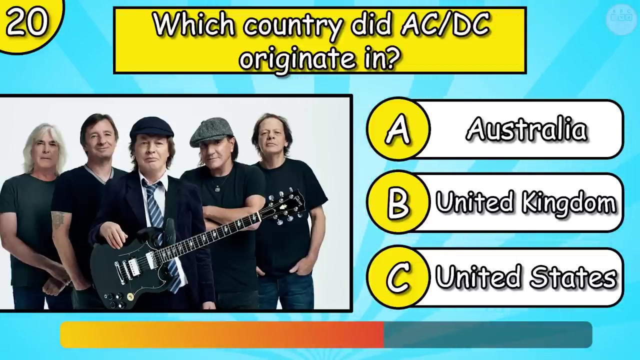 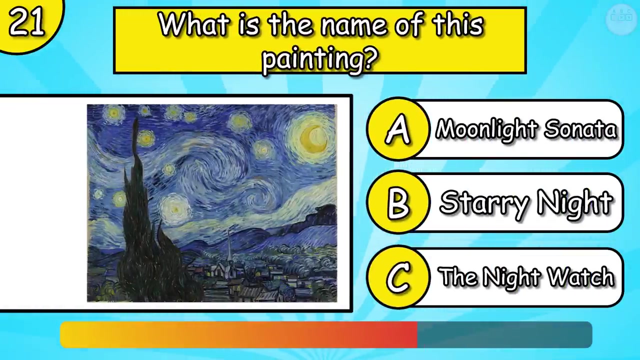 If you don't want to be offended, please go to wwwmicrosoftcom. There are several other forms of gender dictionaries to choose this and similar. How many pyramids of Giza were made? Which country did ACDC originate in? What is the name of this painting? 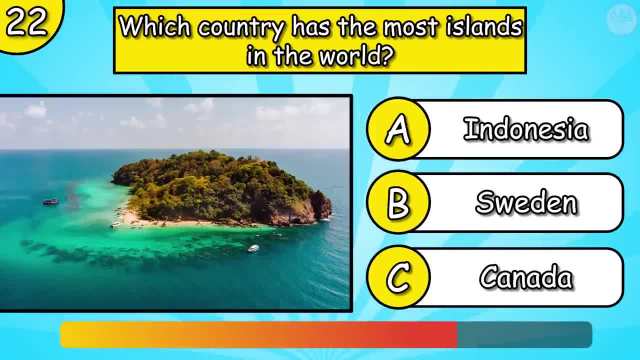 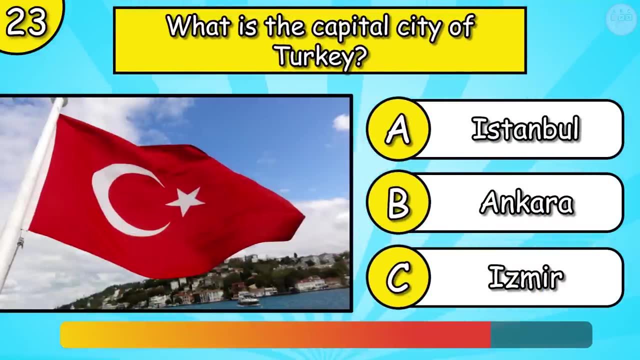 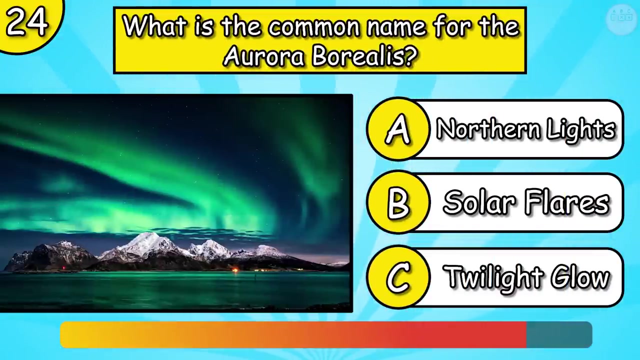 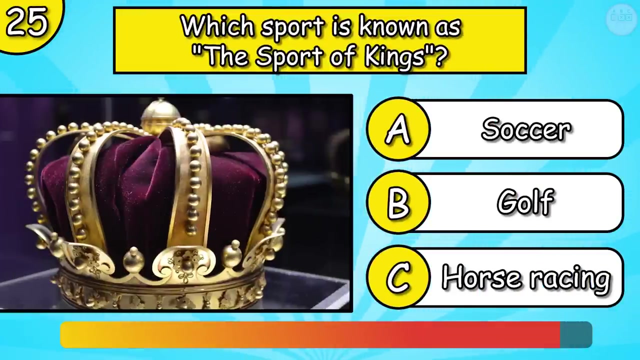 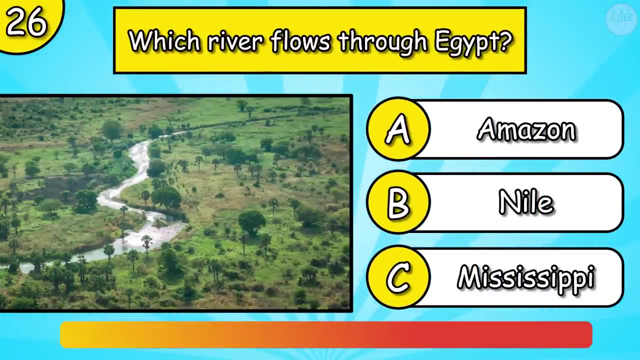 Which country has the most islands in the world? What is the capital city of Turkey? What is the name for Aurora Borealis? Which sport is known as the sport of kings? Which river flows through Egypt? Which river flows through Egypt? What is the name of the land of Egypt? 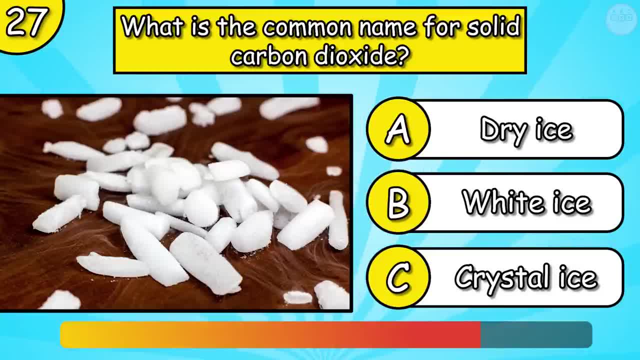 What is the common name for solid carbon dioxide? What is the common name for solid carbon dioxide? What is the common name for solid carbon dioxide? Who is this athlete? I don't know him. Okay, okay, Let's go. Let's go. 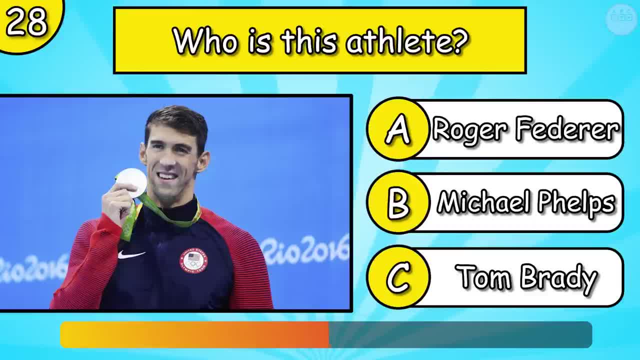 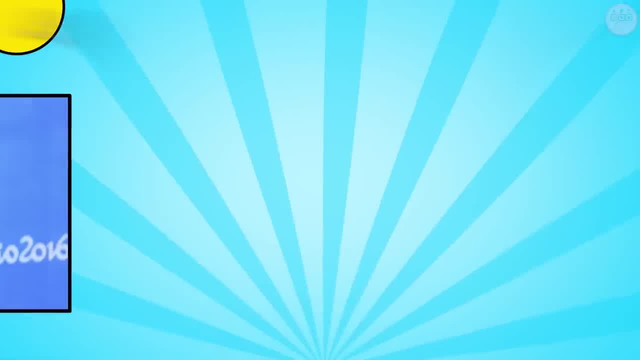 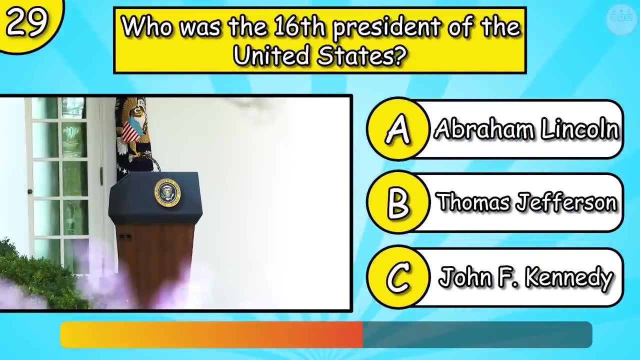 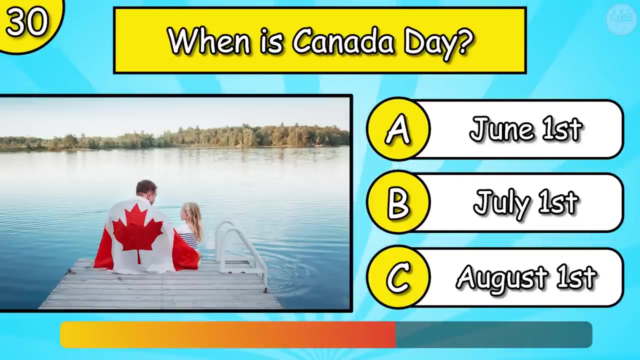 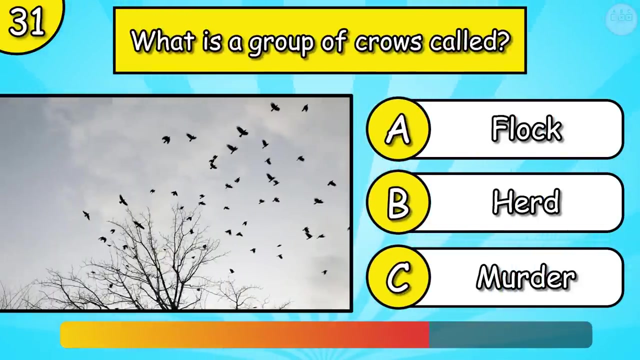 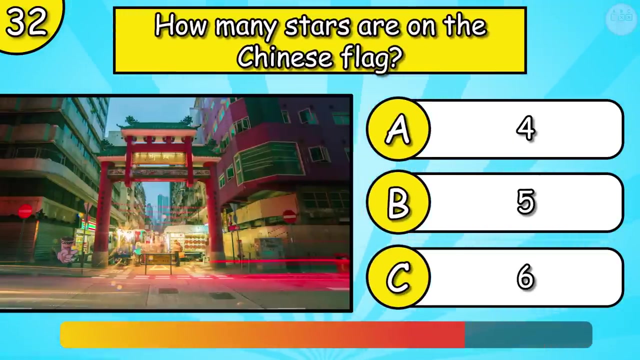 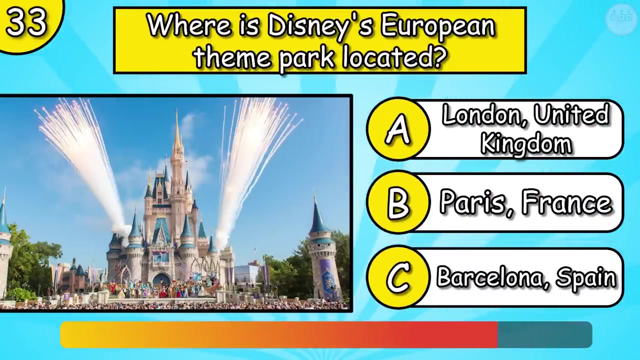 Okay, Okay. Who was the 16th President of the United States? When is Canada Day? What is a group of crows called? How many stars are there in the sky? How many stars are on the Chinese flag? Where is Disney's European theme park located? 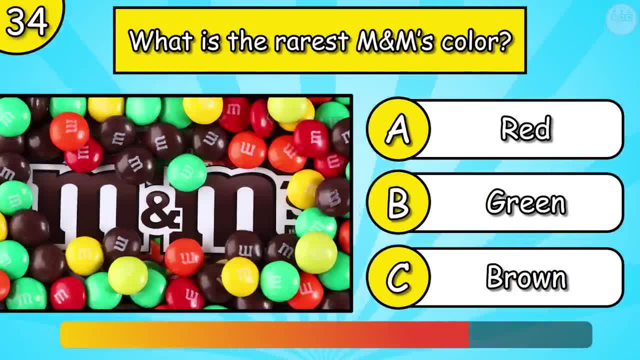 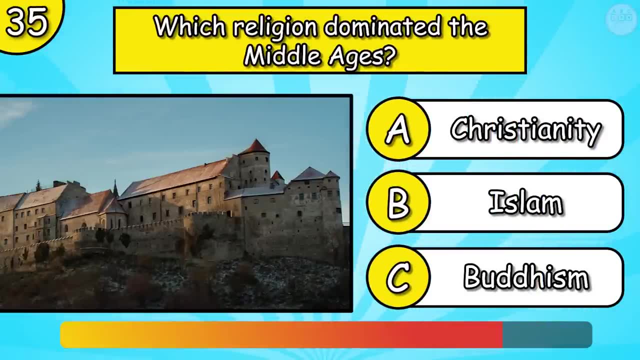 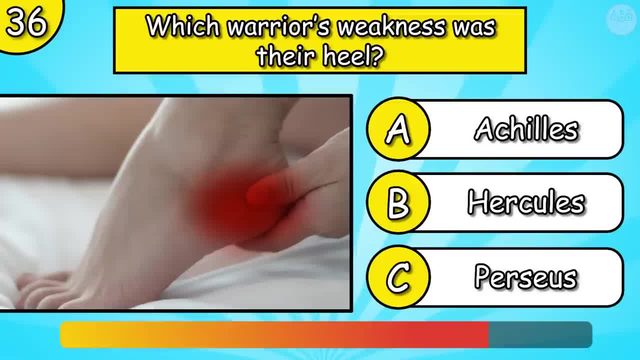 Which warrior's weakness was their heel? Which warrior's weakness was their heel? Which warrior's weakness was their heel? The Elrin Five, The Elrin Five. How many animals are there? How many colors? How many feathers, How many feathers? 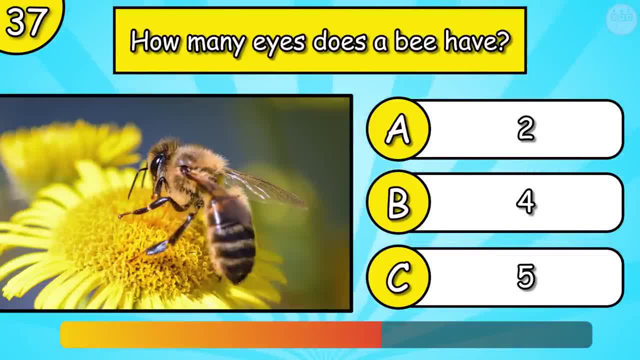 How many soda springs? How many wolverine feces are there in the bluetooth ice feel? How many eye saliva does the bee have? How manyhews does the bee have? Who wrote the novel Dracula? Who wrote the novel Dracula?